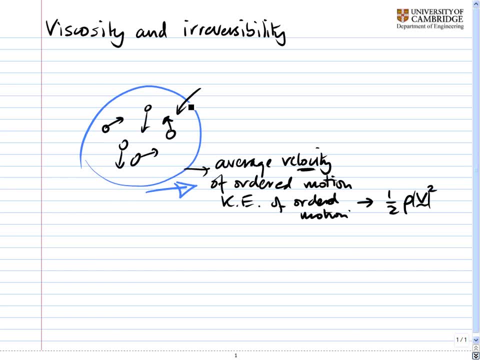 these molecules are moving around so quickly, There's an enormous amount of energy in disordered motion. So we can look at the kinetic energy of the disordered motion. This is measured by the speeds of each molecule And note the difference between the speeds and the velocity. The 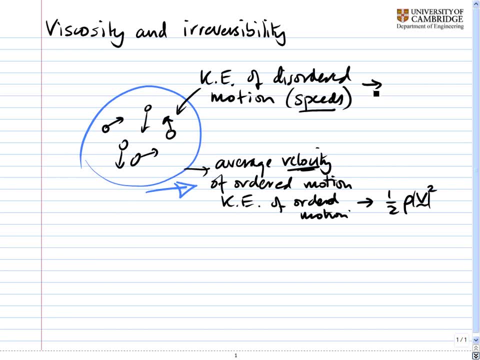 speeds is just how fast they're moving around, And the energy of that is really measured by temperature. Now in thermodynamics you come across the steady flow energy equation, Which says that if you have, going into here, no heat flow and no work being done on this, 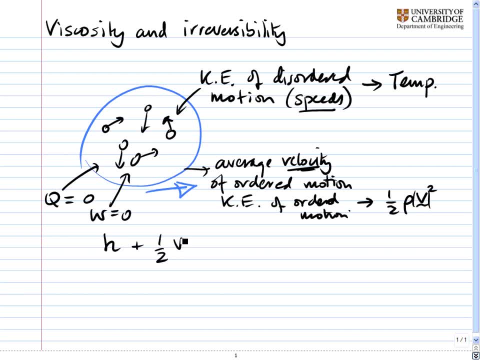 gas, then the enthalpy plus a half v squared is equal to a constant. Now let's imagine we're looking, for the sake of this argument, at something with constant, specific heat capacity. The enthalpy can be written as Cpt plus a half v squared. then the velocity of the ordered 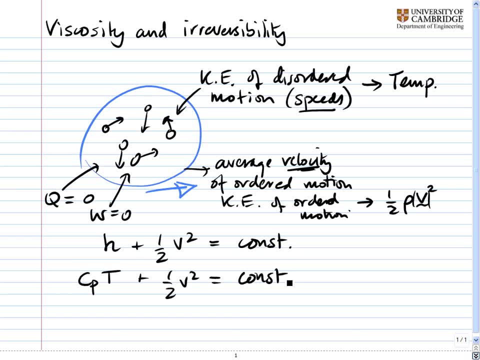 motion is equal to constant. So let's be clear that this resolution is important. Well, if constant- and let's look at what these terms are- the CPT here is essentially, if you like, the kinetic energy of the disordered motion, whereas the half V squared here, by the way, that's per unit mass- is the kinetic. 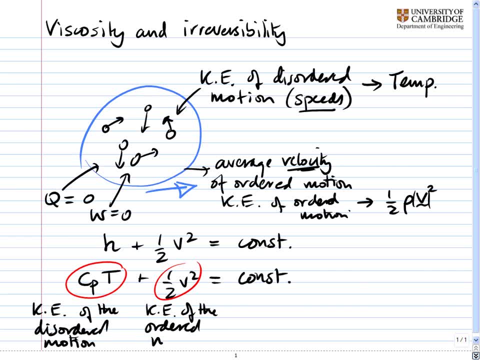 energy of the ordered motion and it's equal to a constant if we're not doing, not adding any heat and not doing any work on that system. so you can see there's a sort of physical explanation there for the terms in the steady flow energy equation and you can also see why if the velocity of the ordered motion 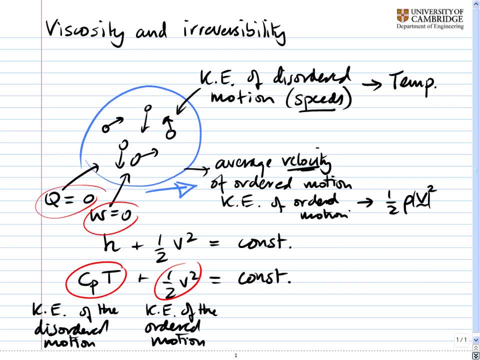 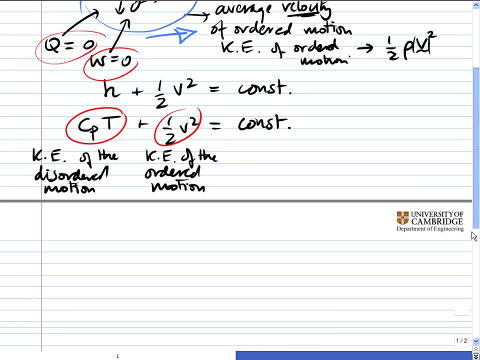 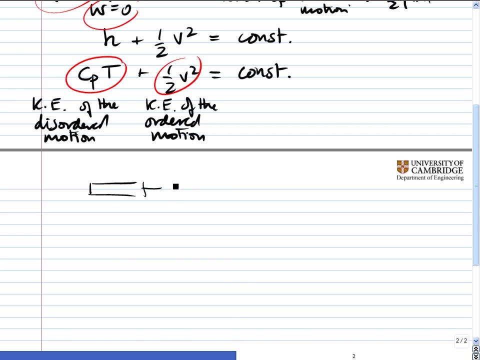 goes down, the half V squared term reduces. then the temperature goes up, which is something that you'll see, or you will have seen in other videos. So let's imagine two layers of fluid, one of them going at velocity V1 with mass m and the other one going with velocity V2 again. 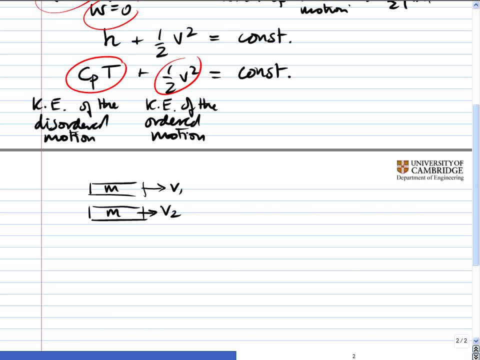 with mass m. Let's think about the kinetic energy of the ordered motion. here it's just a half m V1 squared top one, plus V2 squared for the bottom one, and that's the ordered bulk motion. Now imagine that they mix and that at the 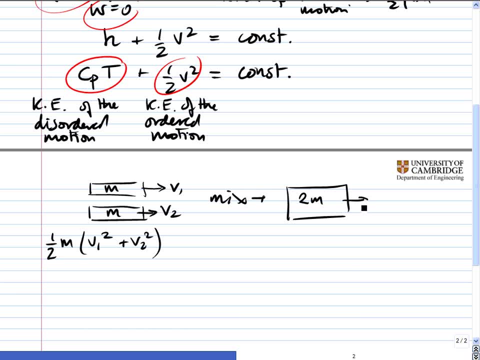 end you've got one quantity of mass: 2m. that's got an average velocity, a velocity now V1 plus V2 over 2, so the kinetic energy of ordered motion here is a half times 2m times V1 plus V2 squared over 2, squared which is 4.. So let's think: 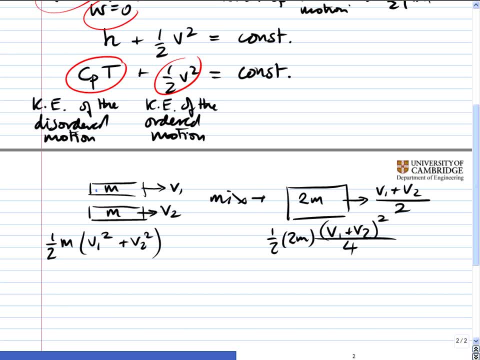 of this kinetically another term- in terms of atoms and molecules. So if you imagine all the molecules that are zooming around in here with an average bulk velocity of V1, we've got all the molecules zooming around in this bit of fluid that have an average or bulk velocity of V2. here they're zooming. 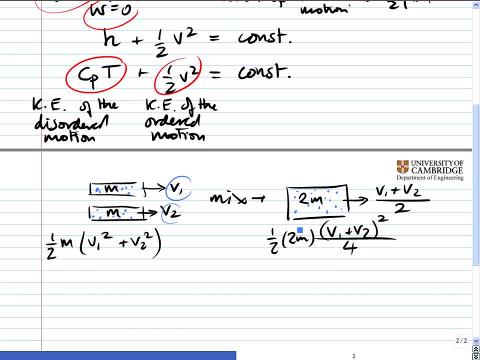 around, as, we'll find out, a little bit faster than they were before, having collided with each other, but they've exchanged their bulk velocity to average it out to V1 plus V2 over 2.. So let's look at the change in the kinetic energy. 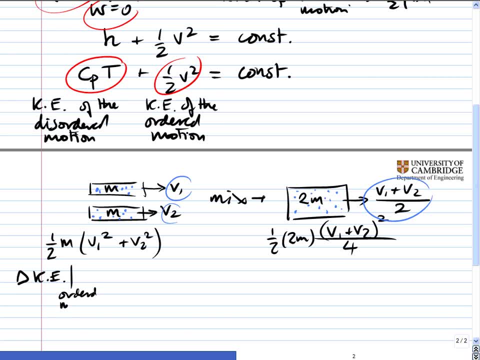 of the ordered motion. Now this is equal to a half m V1 squared plus V2 squared, which is what it was before, minus a half times 2m V1 plus V2 squared over 4.. Now you can do this sum and you'll find that that's equal to a quarter m V1 minus V2 squared. Now, because of the 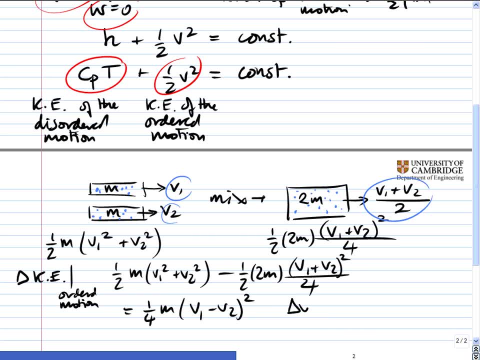 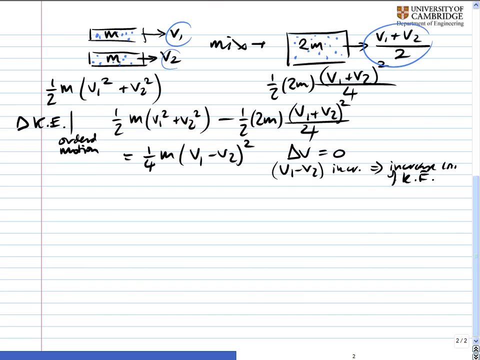 squared term here it's always positive. you'll notice that little check. when delta V is equal to zero, there's no loss in kinetic energy of ordered motion. and as V1 minus V2 or delta V increases, we get an increased loss of kinetic energy of ordered motion. Now where's that gone? Well, of course we know from the steady.